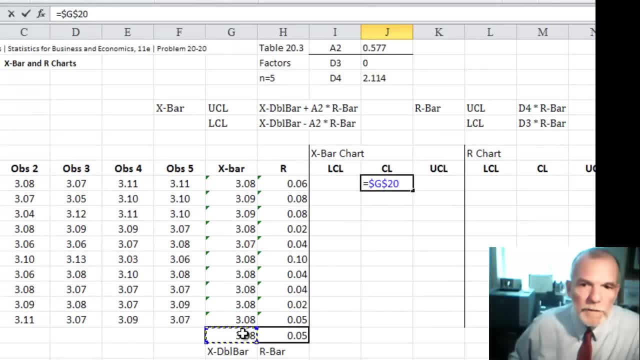 double bar and use the F4 key to make that a fixed reference. Copy it down to the page. Then let's go ahead and do the same thing with the range control chart. The link is R bar, Again F4 key, And then copy it down the page. Okay, so now let's find the lower and upper 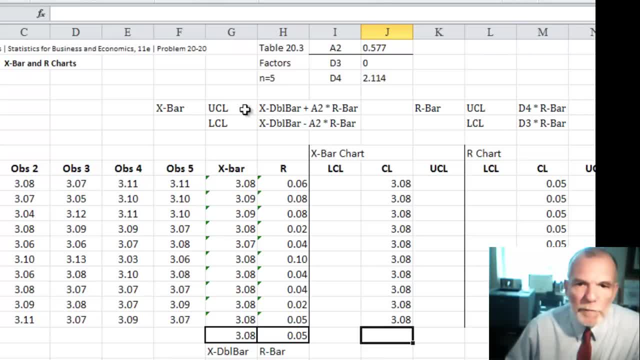 control limits for the X bar chart. You can see it's our X double bar, plus or minus the constant a2, which in advance. I found these constants from a table. The table is very commonly available. It's indexed by sample size, n, which would be 5.. There are five observations, and so for n equals 5, a2 is 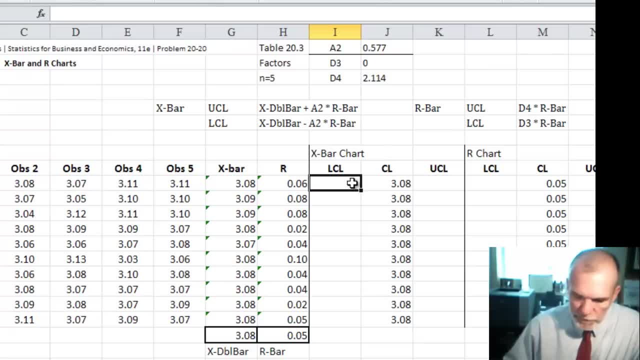 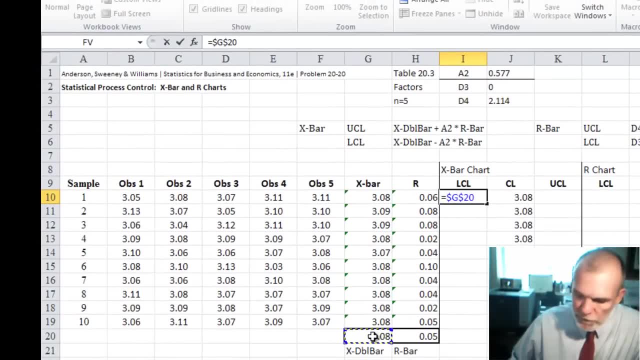 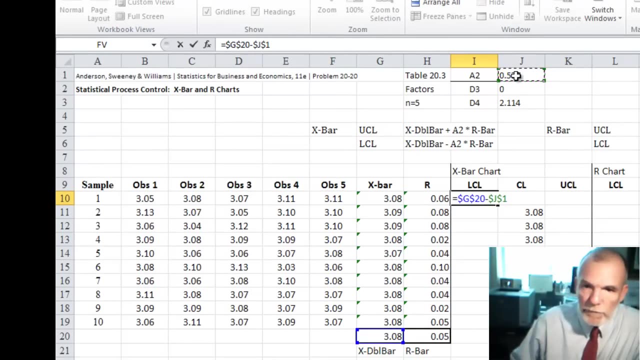 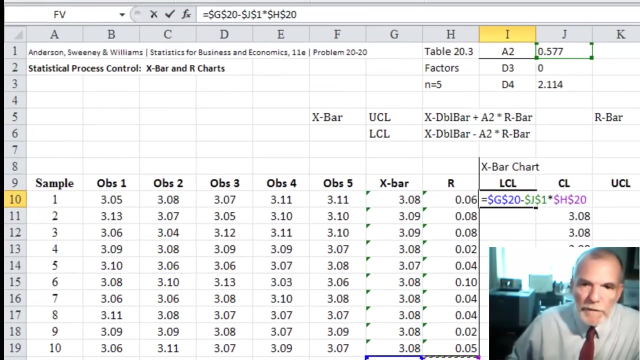 this way 0.577.. So I can just say: equals X, double bar. Freeze that and minus the constant a2, and freeze that and multiply it. times R bar. and by freezing each of those references the lower control limit is going to be a horizontal line, so it should have the same value and all those 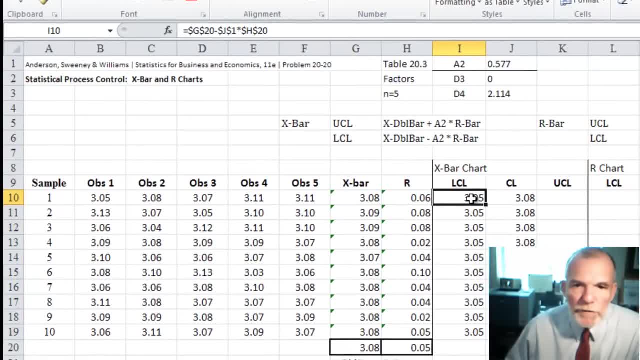 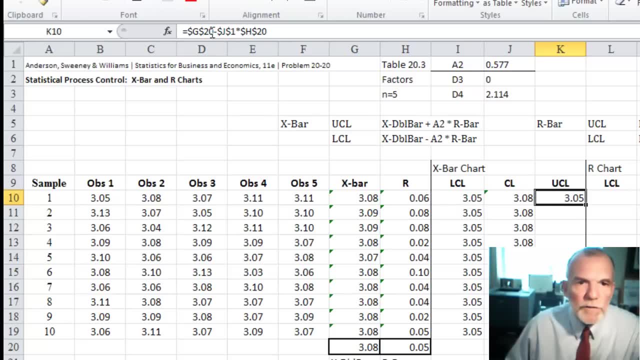 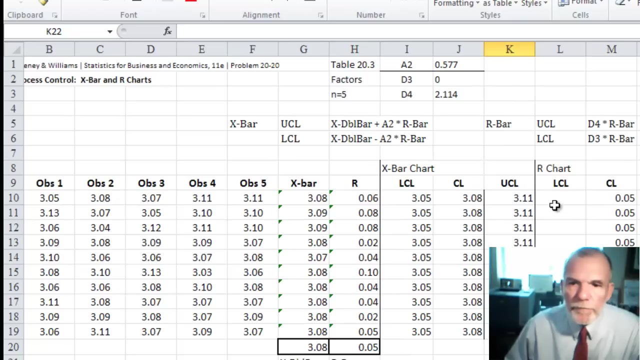 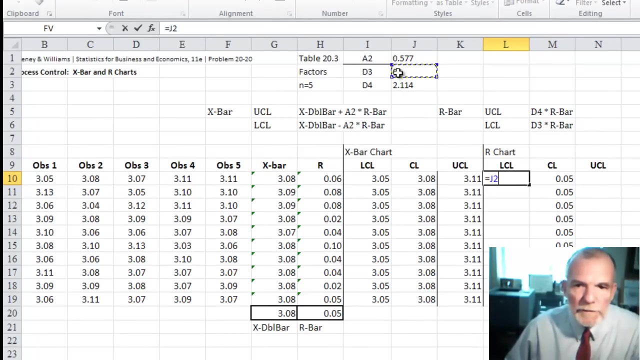 And we could just copy this over and then change the minus to a plus and then copy that down and that would give us our upper control chart limit. For the range chart, lower control limit is D3 times R bar, Again from the same table of constants. I looked up and found this value based on sample size n. 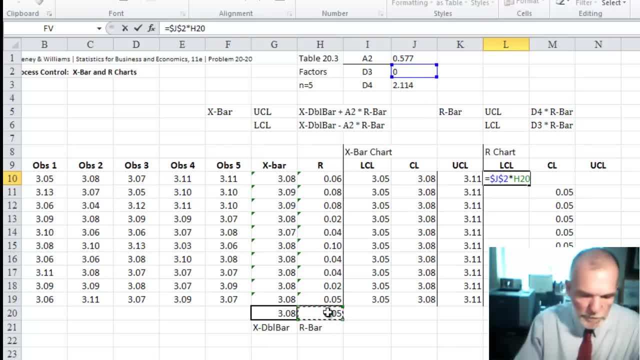 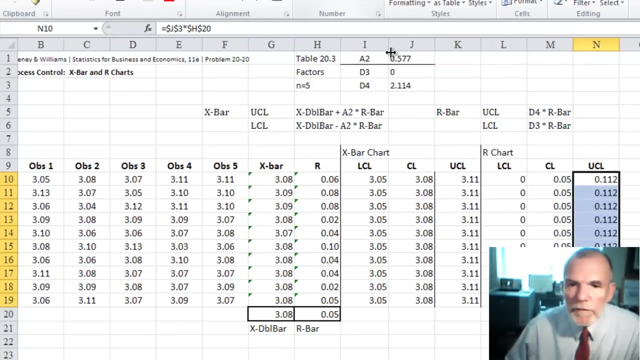 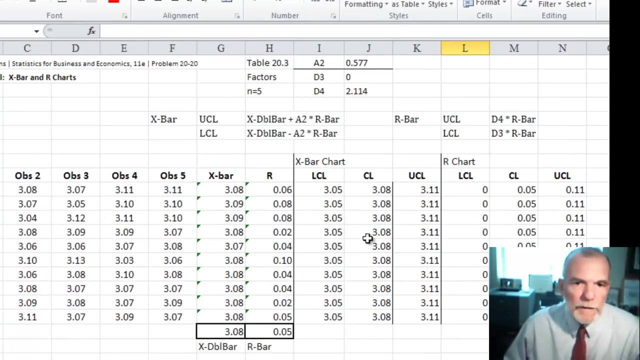 and then multiply that times the R bar and just copy it down and then for the upper control limit equals the constant D4 fixed reference times R bar- fixed reference And then we can copy this down. Now we have the values for creating the charts and so if we were to highlight this X bar, 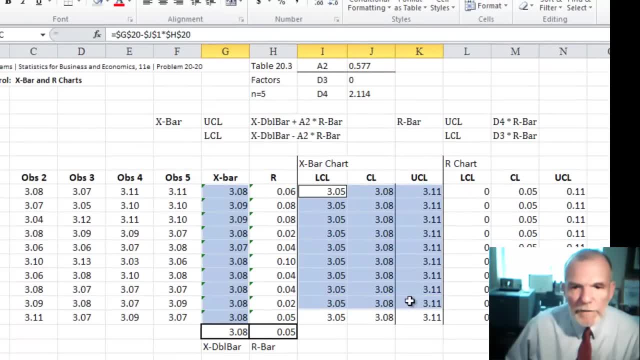 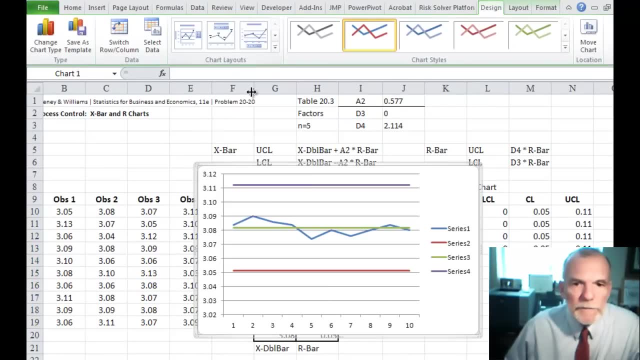 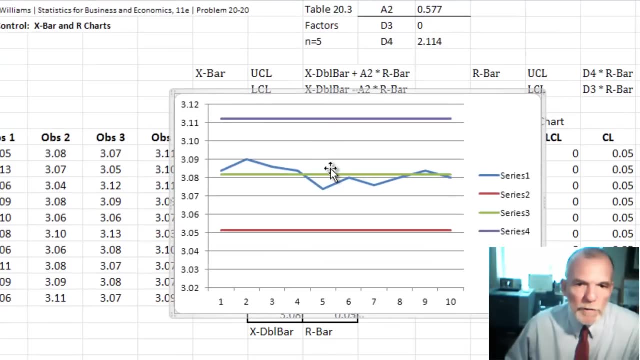 range and then highlight the control limit range and go to insert and line and then we would get the beginnings of creating this X bar control chart. as you can see the upper center line, lower control limits and then our value for X bar. 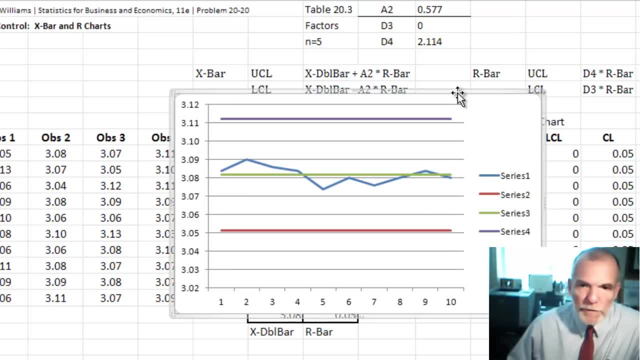 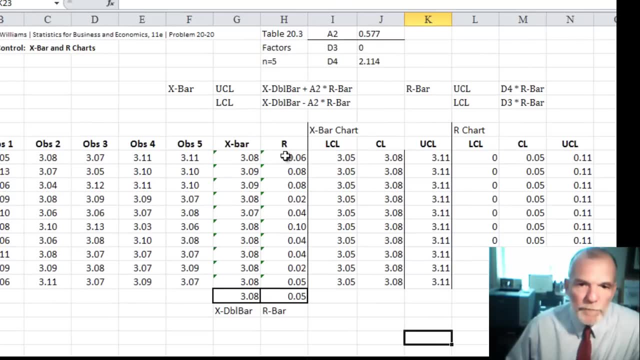 X bar chart. the name of the chart tells us what's plotted on the chart. In a similar way, we could chart the range chart, highlighting the range and the set of three columns here. That's it. It uses Excel to create X bar in our control charts. See you next time. 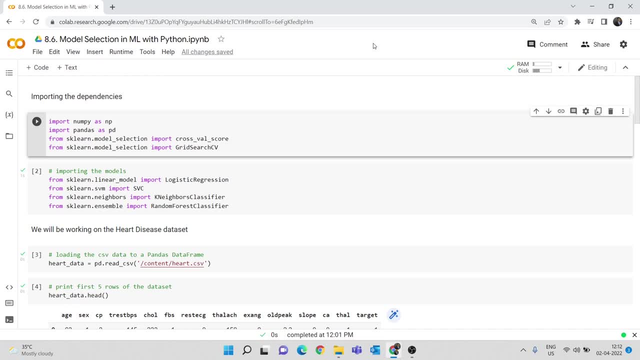 Hello everyone, I am Siddharthan. Currently we are in the 8th module of our hands-on machine learning course and in this 8th module we are discussing about the topics such as cross validation, hyperparameter tuning, model selection, etc. and in my previous video I explained. 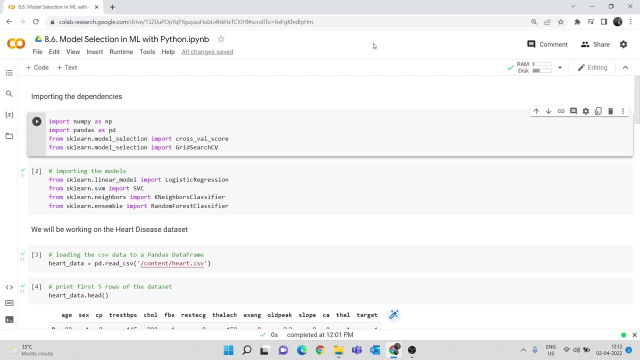 you what are all the different factors that we have to consider while choosing the right model for a machine learning problem, and we have also seen for which kind of dataset we have to use which kind of model, and so on. and in today's video let's try to understand.